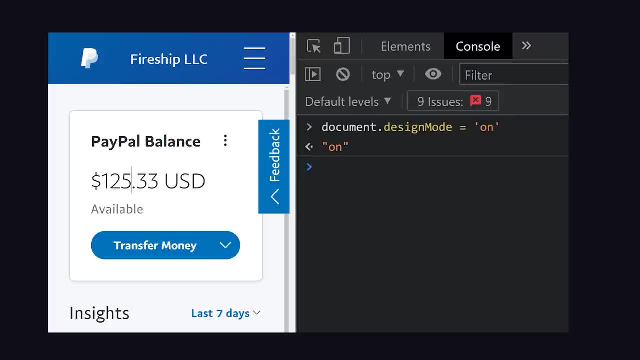 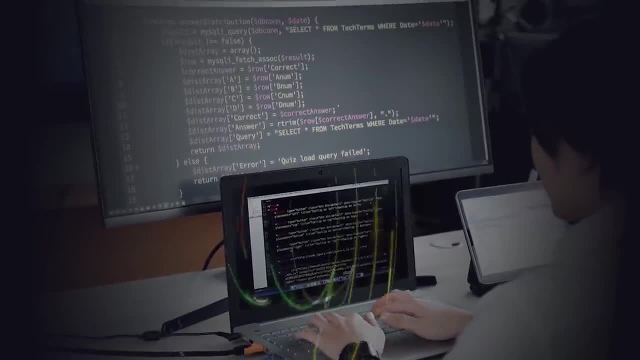 of code to turn the document's design mode on. We can now modify any text in the webpage itself, like the bank account balance. As developers, we tend to take a lot of technologies for granted, one of which is the web browser. Not only is it one of the most important technologies for 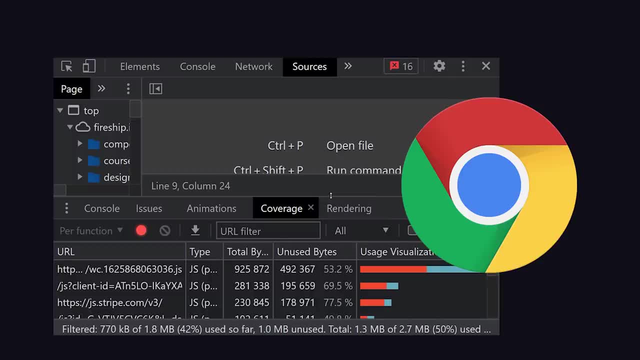 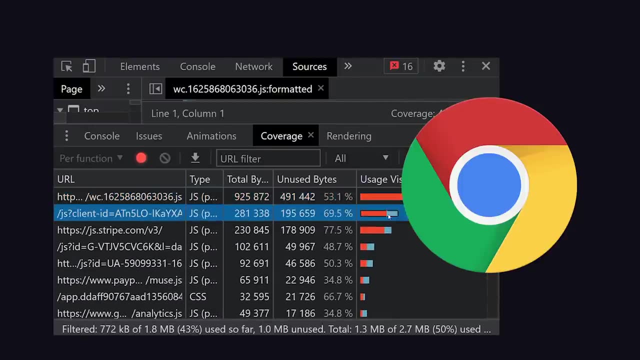 all of humanity, but modern browsers contain all kinds of awesome developer tools that were unimaginable 10 years ago. In today's video, we'll look at a ton of features and tricks in your browser's dev tools that you probably didn't know exist and will make your life. 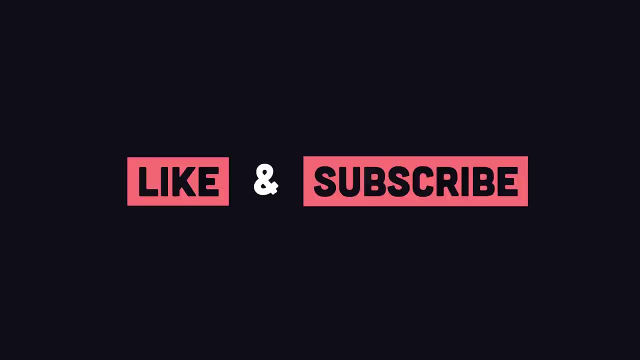 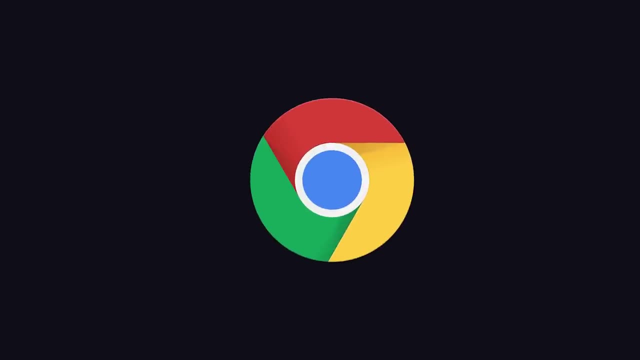 much easier as a web developer. First like and subscribe to keep this content coming. Then add your own pro tip to the comments and I'll pick one of them to win this free t-shirt next week. I'm going to focus on Chrome DevTools in this video, but Firefox also has an awesome. 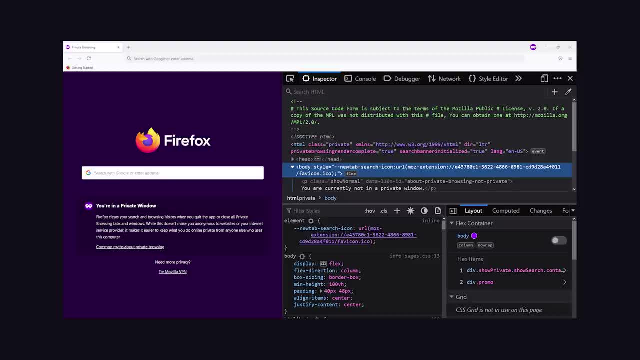 suite of dev tools, and most of the tricks I'll show you apply to both browsers, And if you're interested in learning more about Chrome DevTools, you can click the link in the description. And if you use Edge or Brave, they're both based on Chromium, so everything. 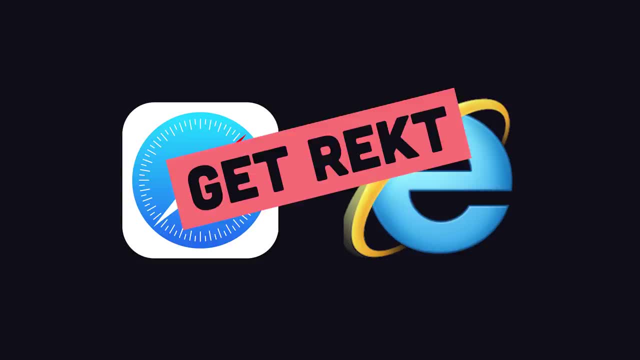 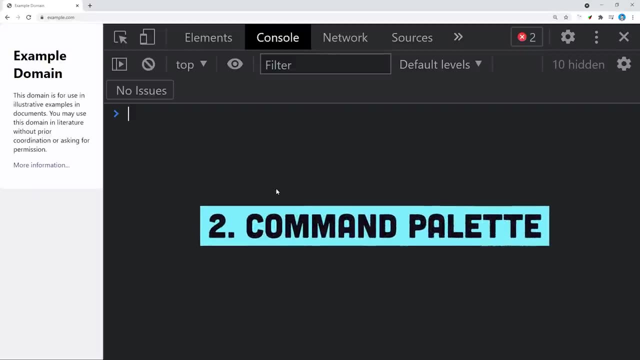 applies there as well, And if you use Safari or Internet Explorer, may God help you. First we need to open up the console, which we can do with the Ctrl, Shift- J shortcut. What you may not know is that Chrome has a command palette, just like VS Code, that you can access. 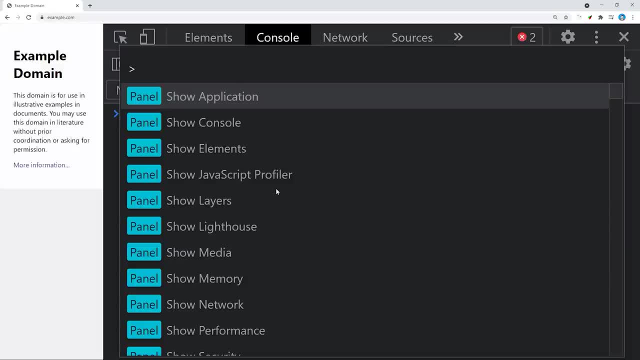 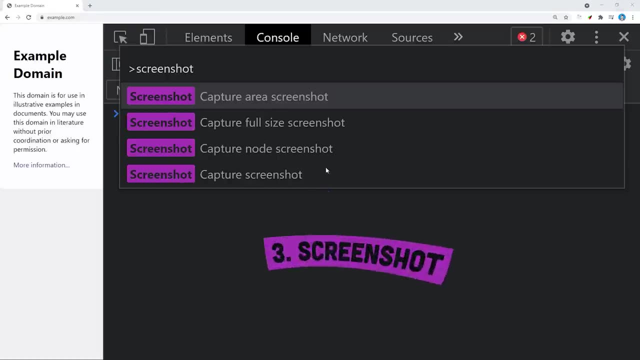 with Ctrl P, Type in angle bracket and that will give you a list of every command at your disposal in the dev tools. A useful one, especially if you want to show off your bank account, is screenshot, which allows you to screenshot an entire page. a custom area. 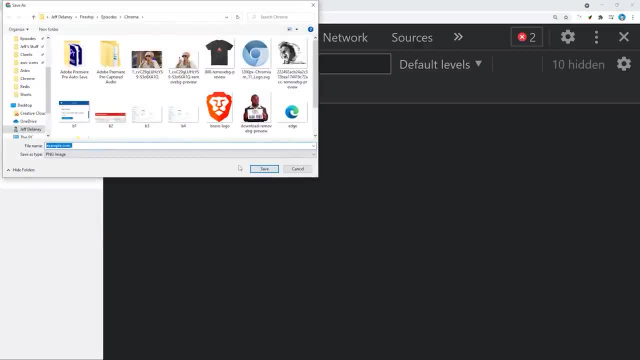 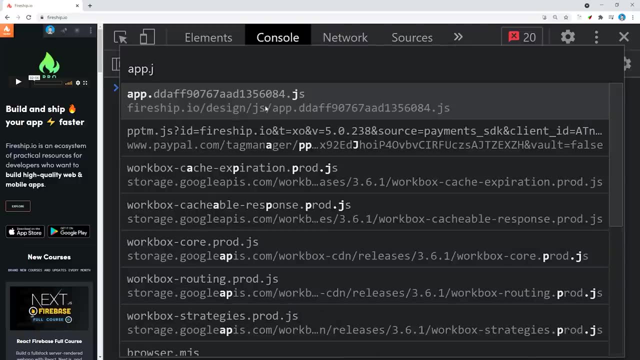 or an individual DOM node. But if we go ahead and open up the command palette again, you'll notice it provides a big list of files. These files are the actual HTML, CSS, JavaScript and images loaded by this web page. When you click on one, 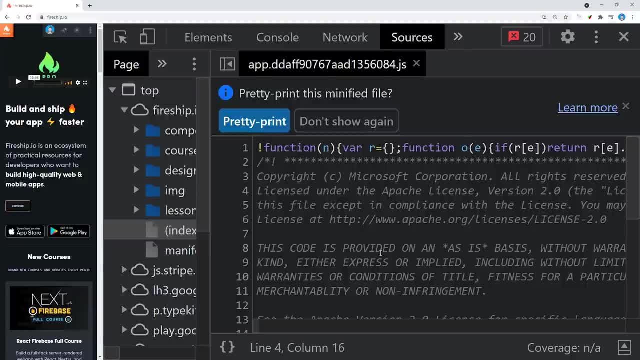 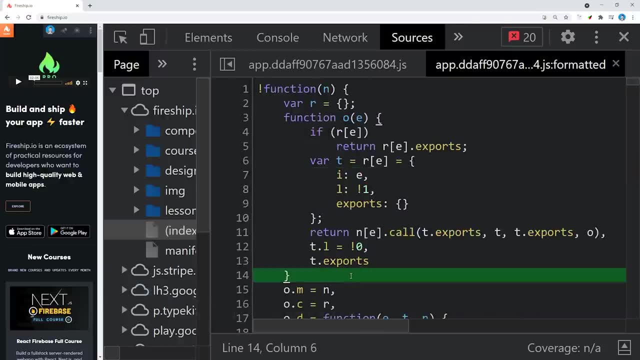 it takes you to the sources tab where you can actually edit and inspect the file In production. it's likely minified, so click the pretty print button to make it look nicer. But here's something you didn't know. In the bottom right corner you'll see the option for. 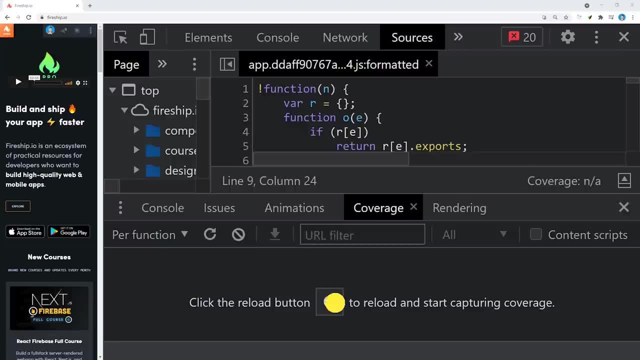 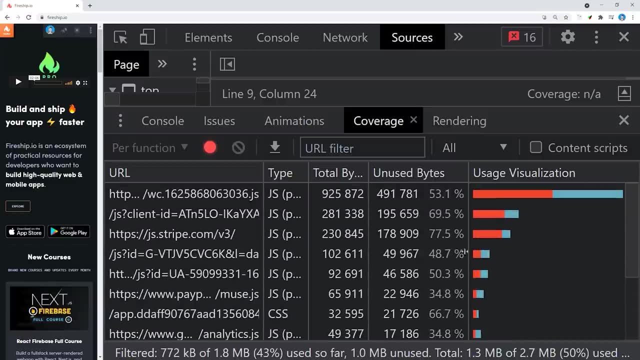 coverage, which will bring up the coverage panel, And this will tell you exactly how much you are contributing to the visual elements on this page. Red bars indicate unused or dead code. that may be making your app slower. You might want to go verify that that code is actually required in. 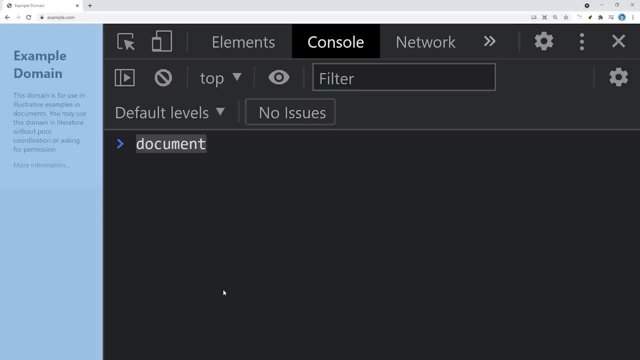 your production bundle. Now, if you want to execute some JavaScript code in the browser, you can do that from the console. You'll likely be using a command like Document Query Selector to grab an element from the DOM, But web developers have always felt that that's way. 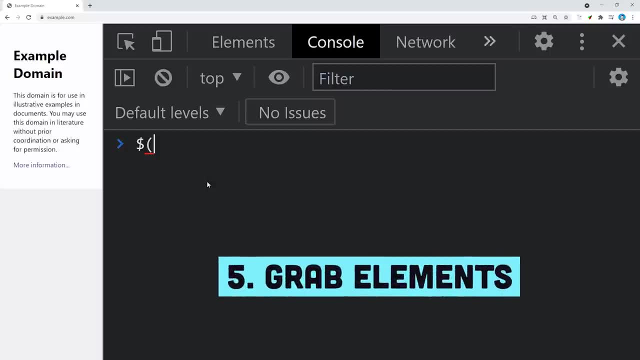 too much code. Instead, use a dollar sign, just like jQuery, as an alias of Document Query Selector. Or grab multiple elements with a double dollar sign, like Query Selector All. Or, if you happen to have something selected in the elements tab, use $0 to grab the current. 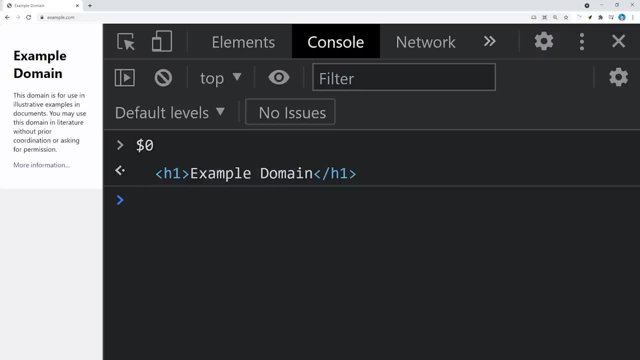 element. Once you've grabbed an element, you may want to see how its value changes over time. You could execute the same line of code over and over again, but a smarter option is to click on the eye icon to pin it to the console as a live expression, where it will automatically update every time. the 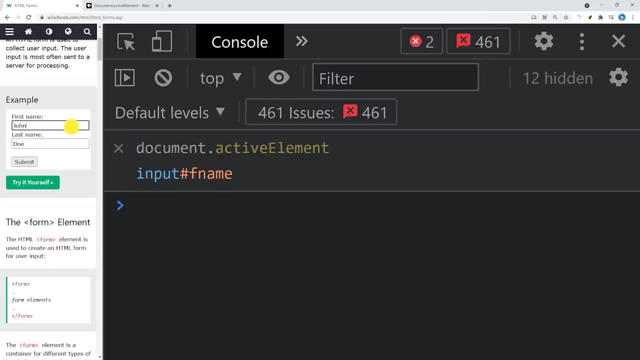 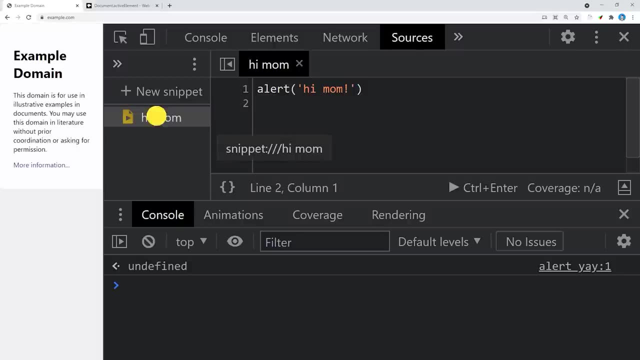 application state changes. In some cases, though, you may want to run more complex code. Open the command palette and create a new snippet. You can write whatever JavaScript code you'd like here. then, when you open up the command palette again and type a bang, it'll be there ready for you to. 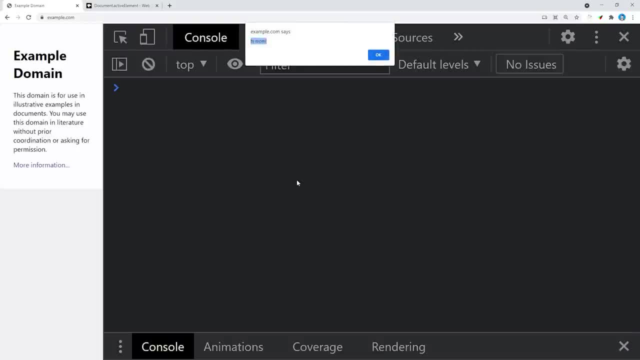 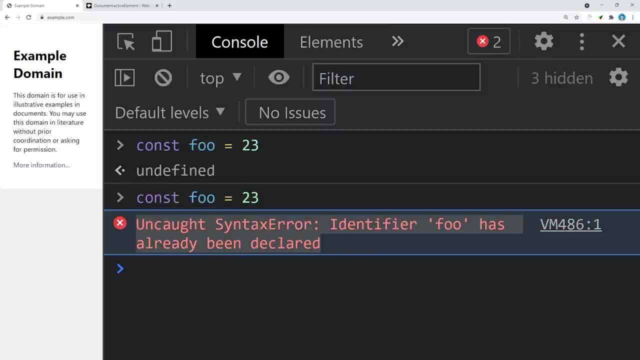 execute whenever you need it. That's pretty cool, but one thing that can be kind of annoying is that when you're messing around in the console, you might want to redeclare the same variable over and over again. Using const with the same name twice would normally produce an error. 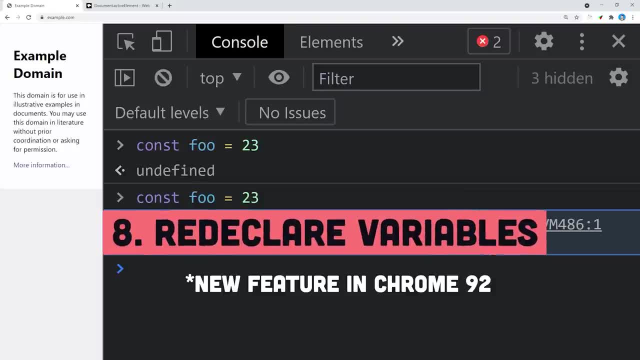 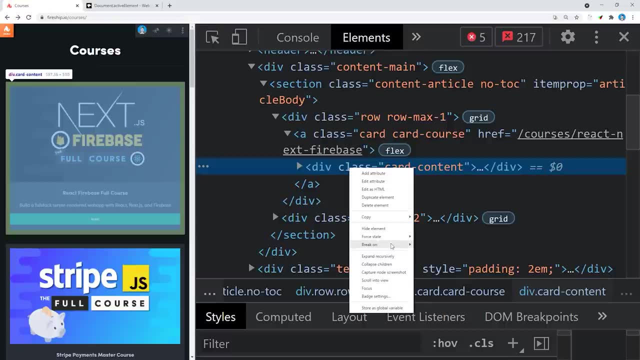 but in the Chrome console it's no problem, because we're just messing around here. JavaScript is one thing, but more often than not I'm using the browser dev tools to debug my HTML and CSS. If I'm illegally scraping a website, I might want to go to their HTML and copy an element. 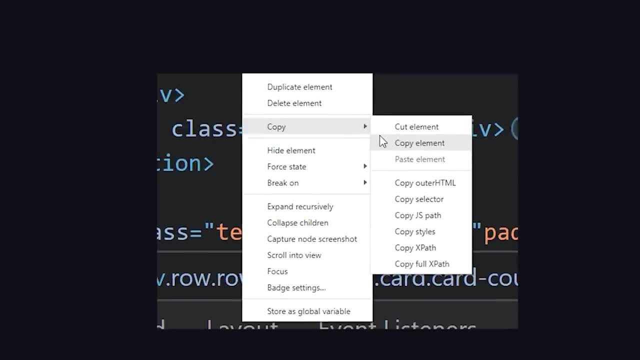 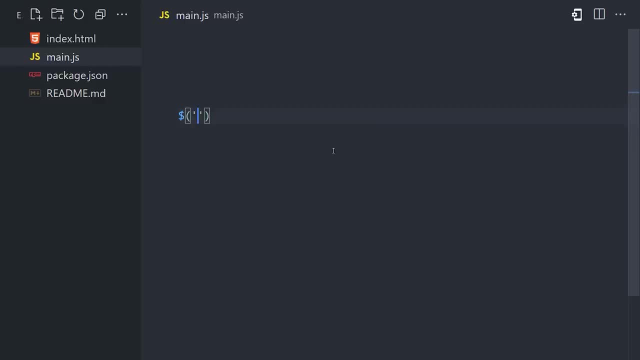 into my own project. I could just copy the element with control C, or I can right click and get a variety of different copy options. An especially useful one is copy selector, because I can then use it to target an element in my CSS or JavaScript Or, if I really like the way, an element. 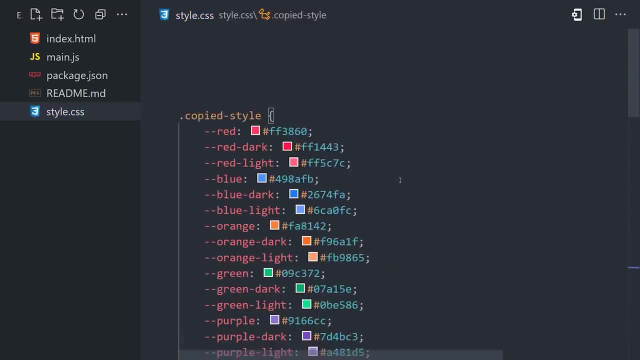 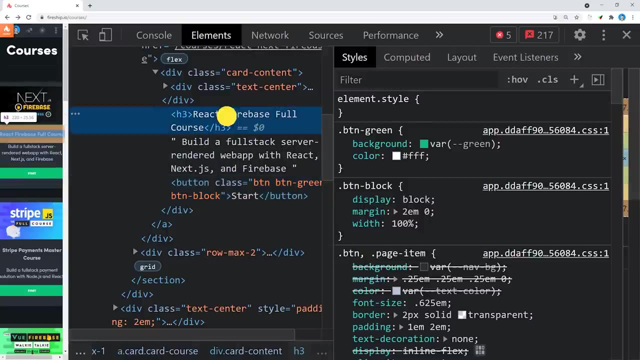 looks. I can copy its styles and paste them directly in my CSS. When you click on an element in the DOM, it will show you all of the CSS styles that apply to it in the styles tab. But what if you want to see the styles when an element is hovered or focused? You can do that by right clicking an. 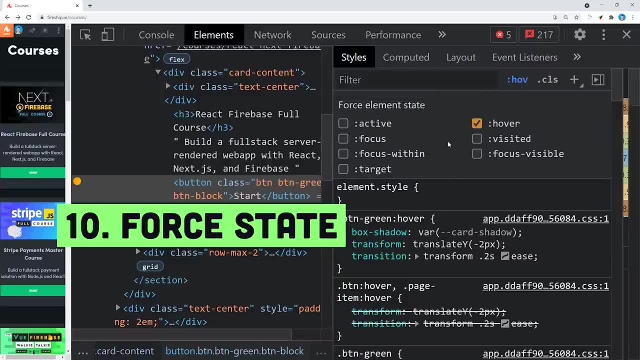 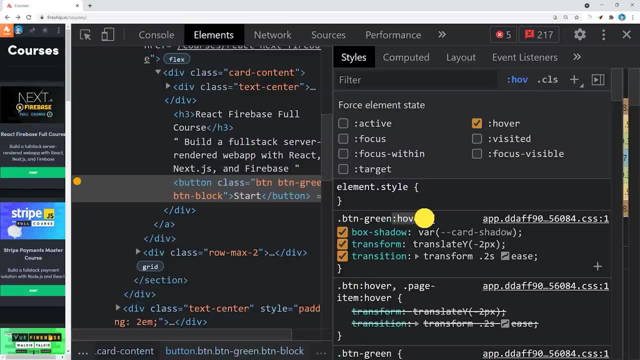 element or from the styles panel you'll see the HOV button to force an element state. That'll cause the element to stay frozen in that state, making it easier to inspect that CSS. That's useful for simple transitions, but you might also have complex animations on a page. The 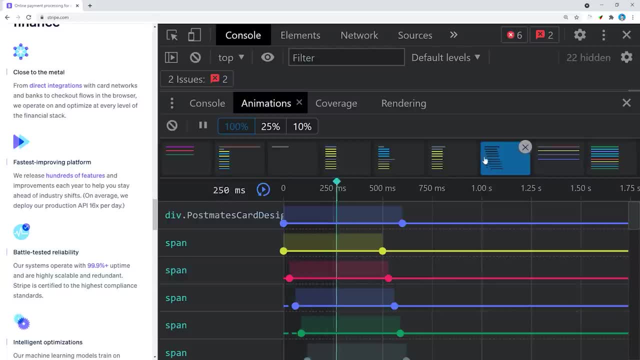 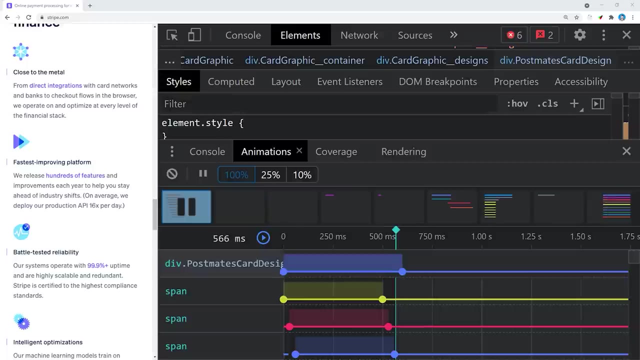 animations panel allows you to record any keyframe animations that are happening on the screen. You can scrub them back and forth slowly and inspect the actual CSS properties that they affect, and is really useful for understanding how animations work on other impressive webpages. However, if you go too crazy with your animations, it may slow down the rendering of the webpage. 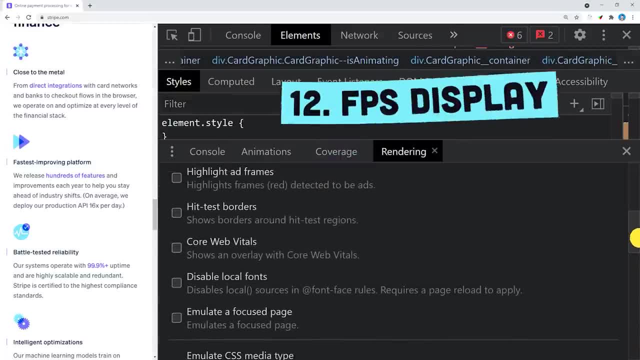 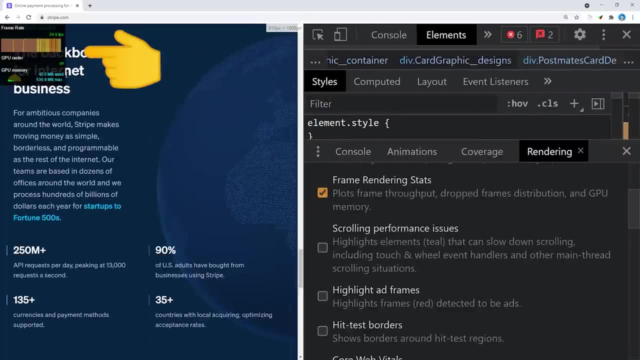 causing jank and just an uncomfortable user experience. The rendering panel is like a heads up display that helps you detect a variety of different issues before they become a problem. If we check the box for frame rendering stats, it will provide data about the frames per second and 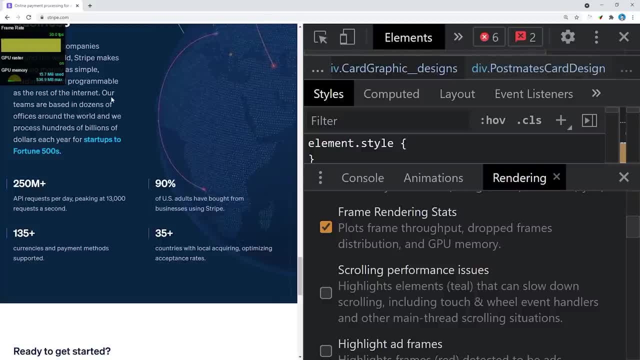 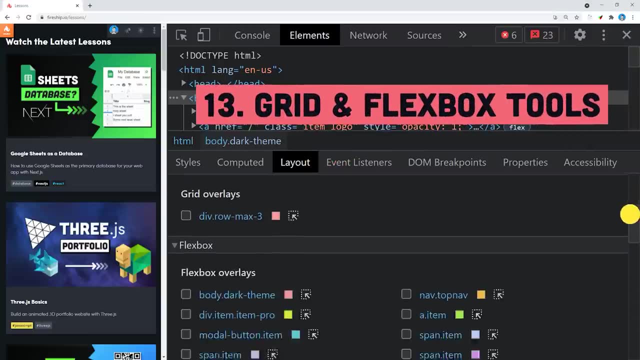 the total memory used on the GPU. Now, CSS is awesome and all, but the best kind of code is the code that you don't have to write. If you're working with flexbox or grid layout, go to the layout tab and draw visual markers. 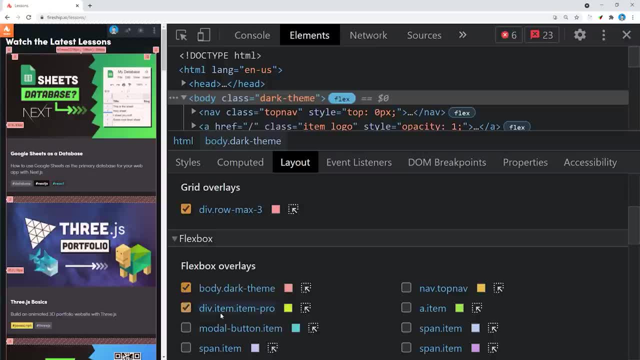 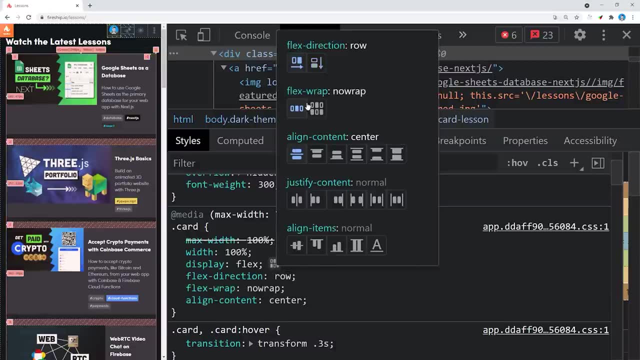 around those elements by checking the boxes that you want to see. Back in the styles tab, if you go to the display property and its value is flexbox or grid, you'll see an icon that you can click on. That brings up a dialog where you can modify the layout without having to memorize. 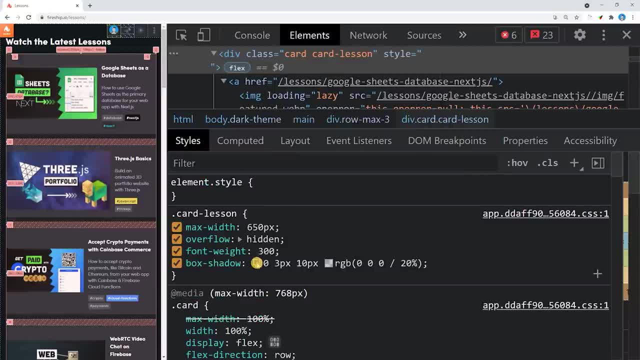 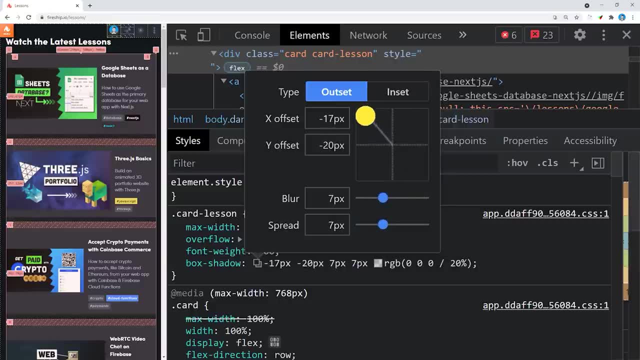 a bunch of confusing CSS properties, And there's also a similar tool for box shadows, which are notoriously difficult to code by hand. But if you'd rather modify your website with something more like an actual design tool, check out the Visbug extension It allows. 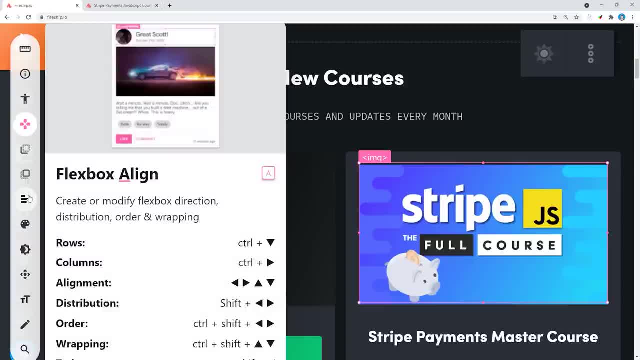 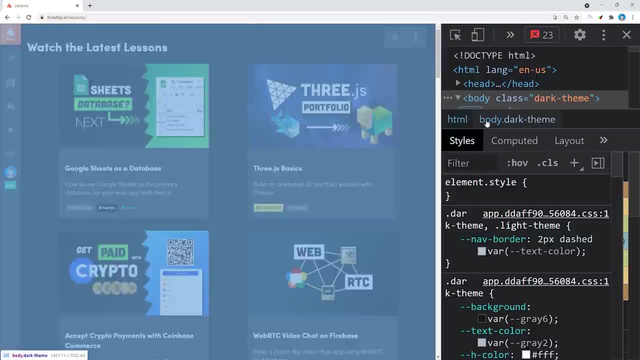 you to interact with the webpage itself and modify its appearance without knowing or understanding CSS whatsoever. Now your design may look good on your machine, but how do you know it's responsive to different screen sizes? You can find out by clicking on the device toolbar. It provides a 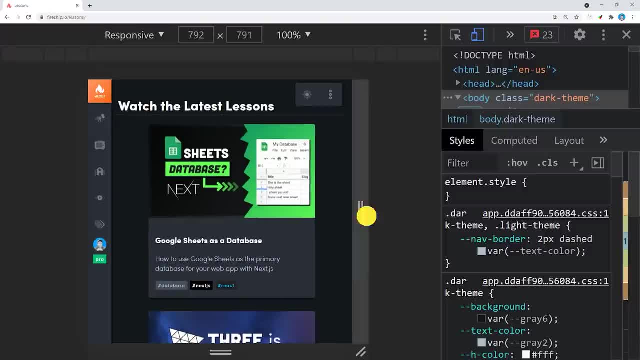 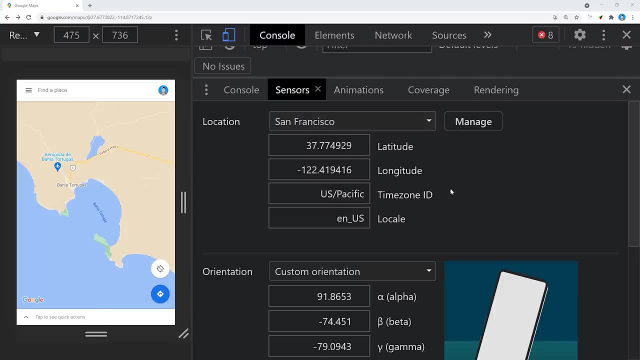 bunch of common screen sizes to choose from, or you can use the responsive option to resize it yourself manually, And you can even throttle the network speed here to simulate low-end devices. But the fun doesn't stop there. If you're targeting mobile devices that use geolocation or motion, you 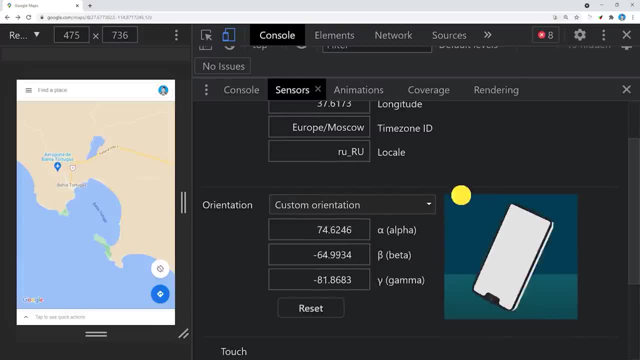 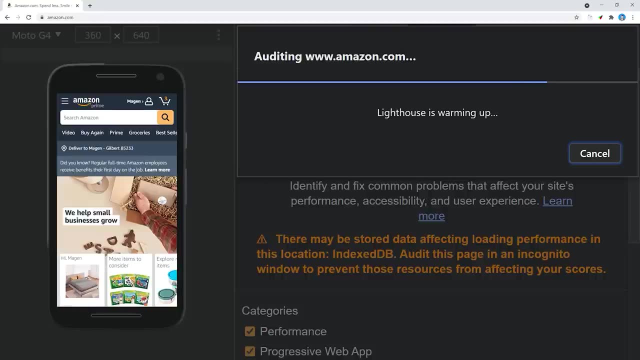 may want to make sure that you're using a mobile device. If you're targeting a mobile device, you may want to make sure that you're using a mobile device that uses GPS coordinates and device acceleration and motion from the sensors panel. If you're targeting mobile users, then you're likely. 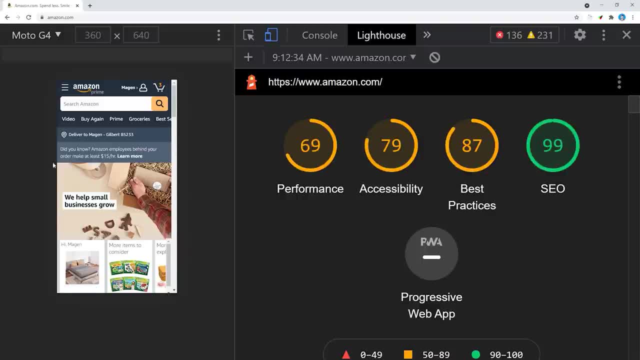 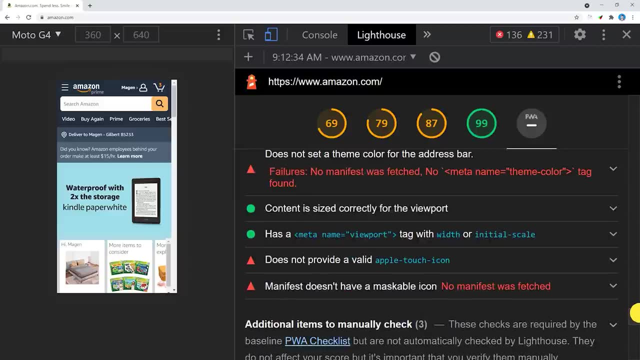 building a progressive web app. The Lighthouse tool will analyze your website for performance, search engine optimization and progressive web app features. If you pass the audit, it means your website can be installed on a mobile device just like a native app, And if you fail the audit, it. 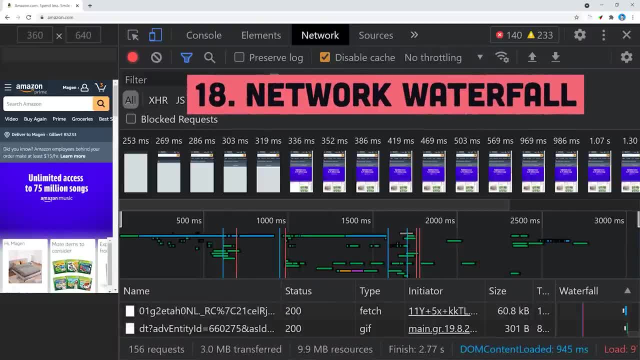 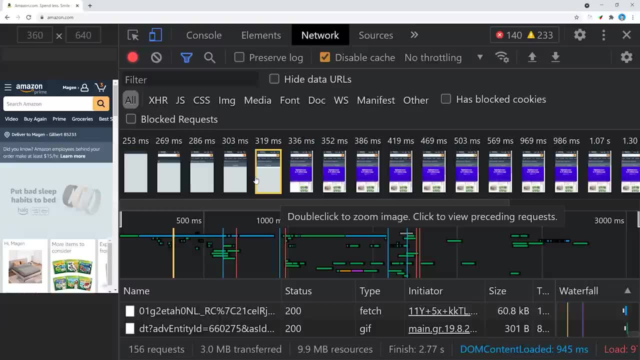 will tell you exactly what you need to address in order to make the experience for mobile users better. You can also use the Lighthouse tool to track your website's content, And that's usually because it tries to load too much JavaScript and CSS. You can inspect exactly how the browser loads. 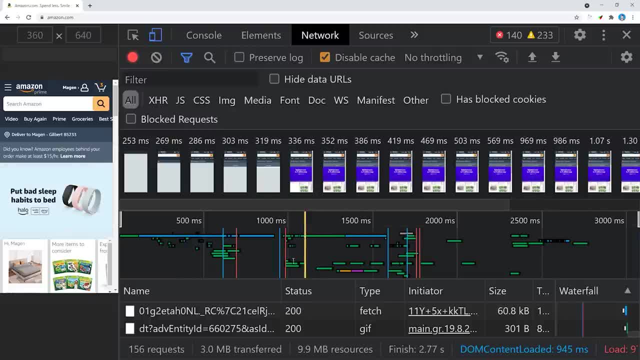 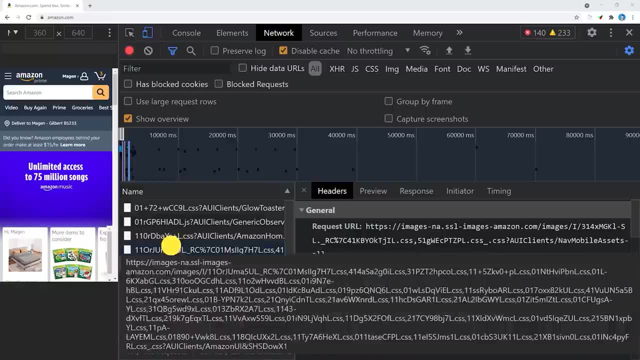 all of your assets. by going to the network tab, It creates a waterfall graphic that shows every request the browser makes and how long it takes to fetch each one of those assets. If you're worried about performance, turn on screenshots to see how your website loads after each request is completed. 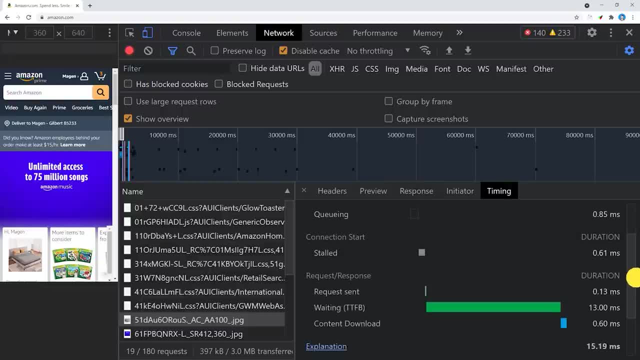 Clicking on an individual item will provide a breakdown of the response body and headers. And if you want to dive really deep into performance, click on the timing panel. It'll show you exactly how the browser loads and how long it took to fetch something. breaking down the timing all the way. 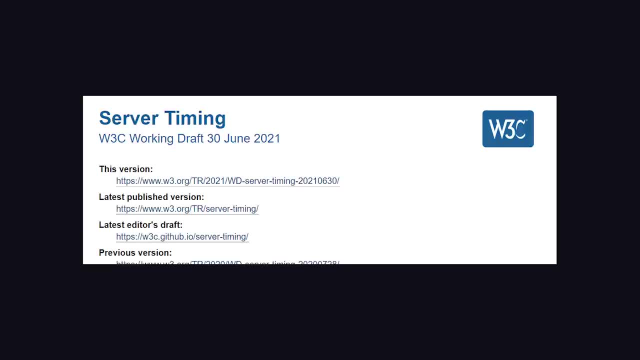 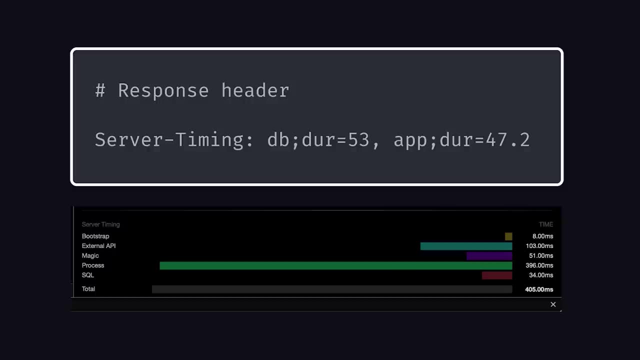 to the DNS level. What you didn't know, though, is that there's actually a server timing API that allows you to pass more detailed information from your server to the browser. When the server timing header is present on a response, Chrome will automatically break that information down in the 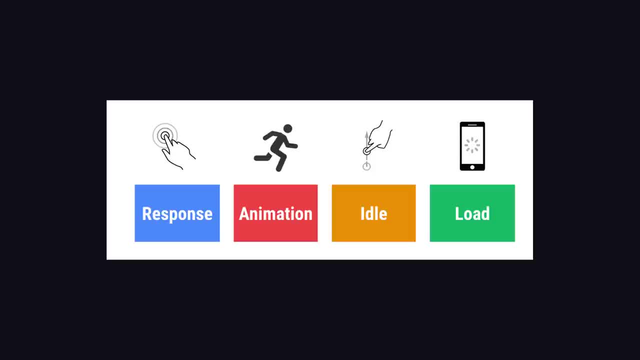 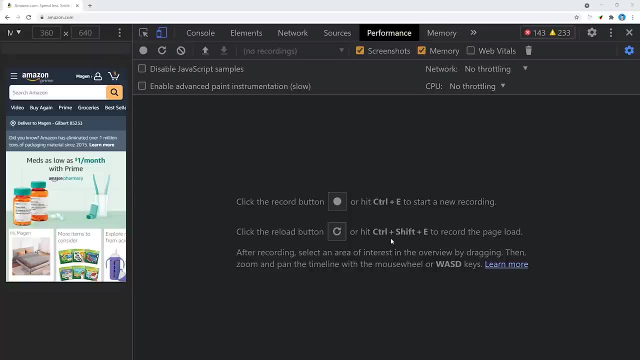 browser dev tools For the end user. there are four main issues when it comes to performance: Response, animation, idle and load. Lighthouse and the network panel can help you debug loading issues, but for the other three we'll need to analyze the 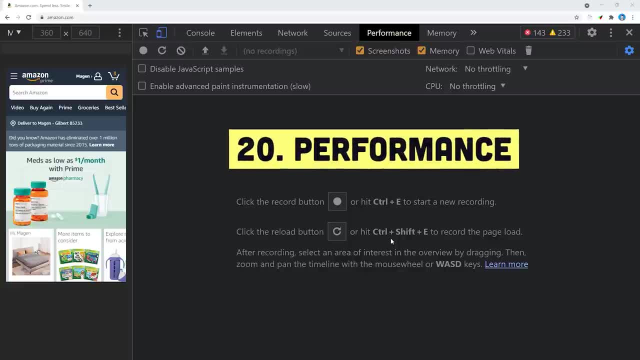 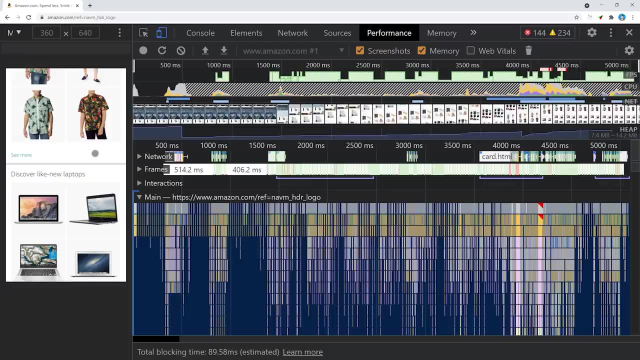 actual runtime performance of our code, which we can do in the performance panel. Hit the record button, then start using your site like an end user. When you end the recording, it'll give you a breakdown of the CPU usage frames per second and the amount of memory. 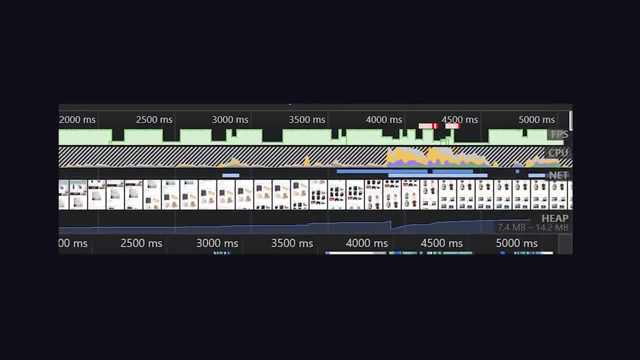 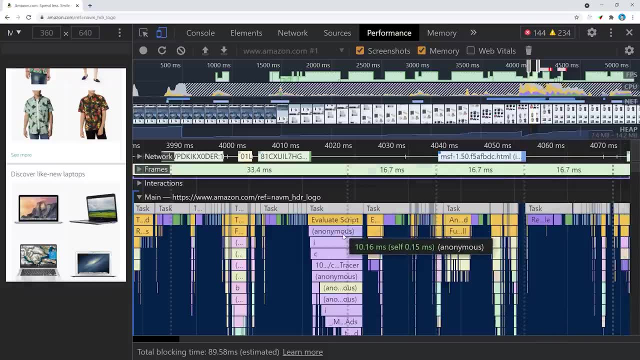 allocated to the heap. If you notice a spike in CPU usage, a drop in frames per second or a jump in memory usage, it might indicate an area of code that needs to be optimized. To investigate further, Chrome has generated a flame chart that breaks down everything that. 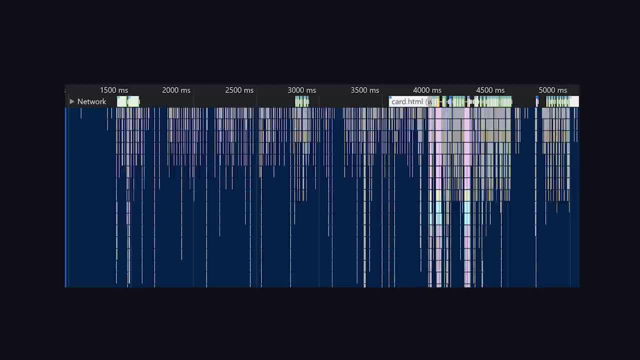 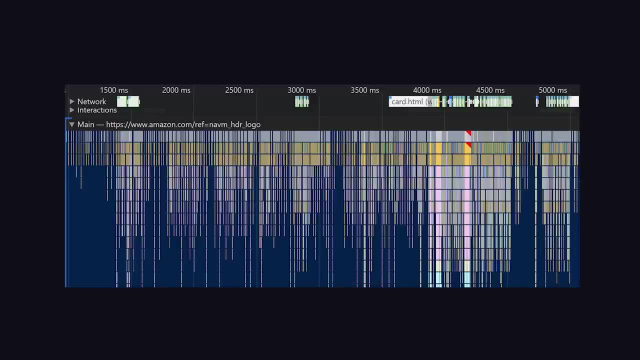 happens on the browser's main thread. In other words, this is how the browser executes your JavaScript step-by-step: The x-axis represents time and the y-axis is the call stack. If the chart is really tall, it's not much of a problem. You might just be calling. 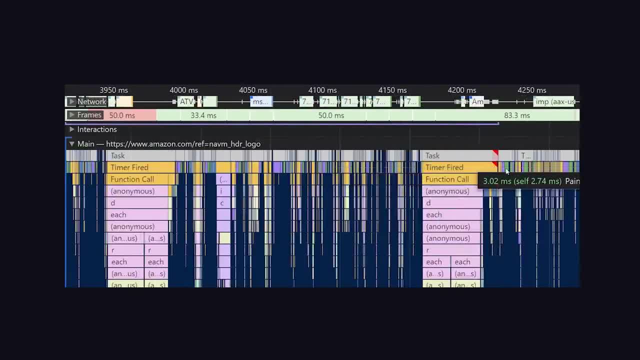 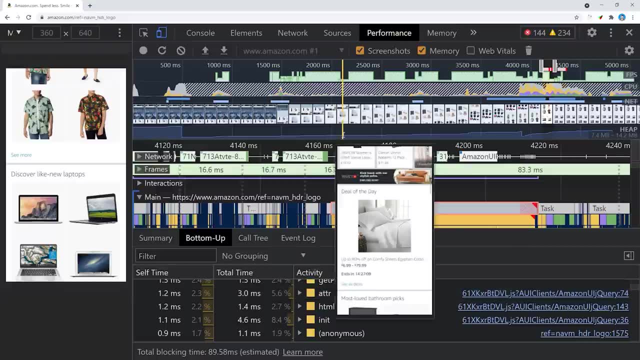 deeply nested functions, But if a frame is really wide, it means that something is taking a long time, In which case you should click on it to investigate why your code sucks in more detail. Now, in some cases, the main thread might be fine, but your code might create a memory leak. 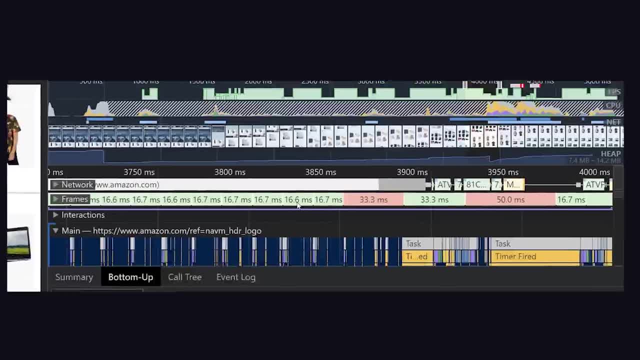 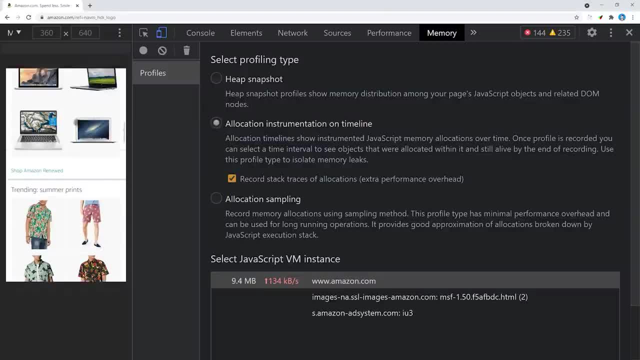 by allocating memory to objects that you no longer need. You can tell you have a memory leak when this blue line gets bigger and bigger. But to investigate further we'll need to create the memory tab. Select the option for allocation instrumentation, then hit the record button.